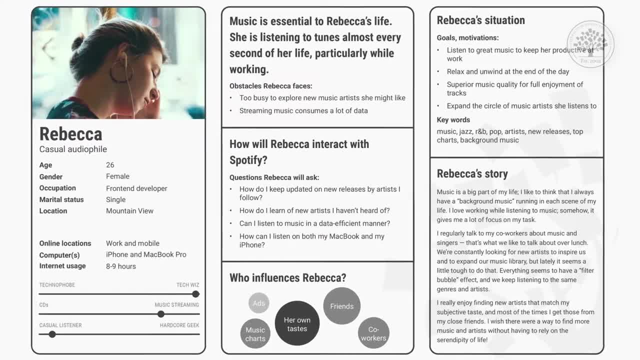 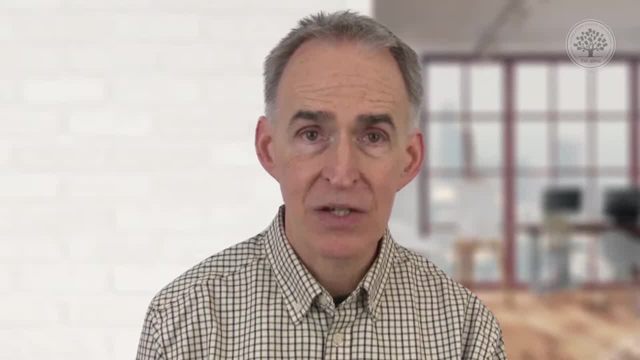 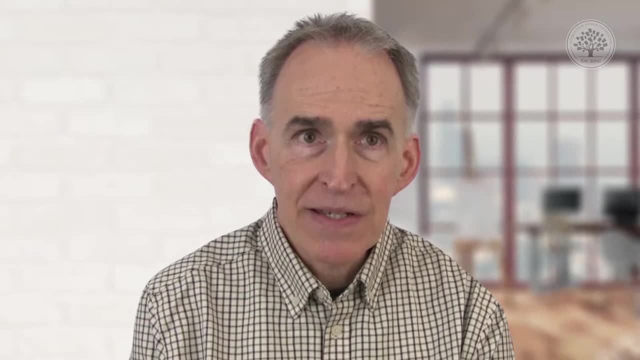 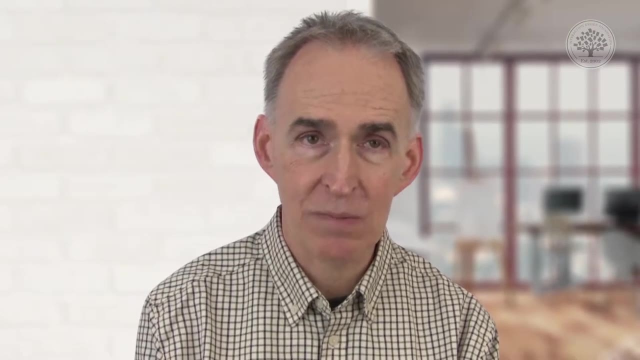 That we replace roles or users with actual names of people, because that gives us a much better chance of promoting empathy, promoting an understanding of their situation and their needs and behaviors. So key features of user-centered design: direct engagement with users. If anybody asked me what the main feature of user-centered design was, that would be my. 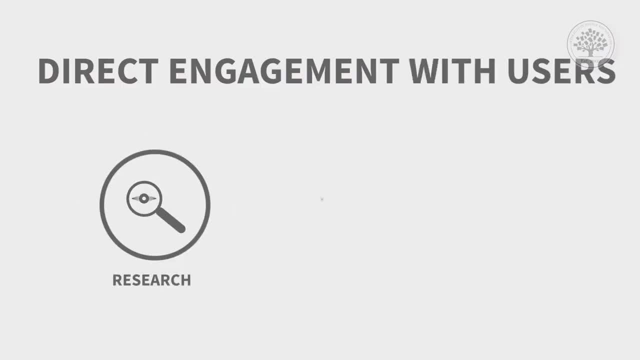 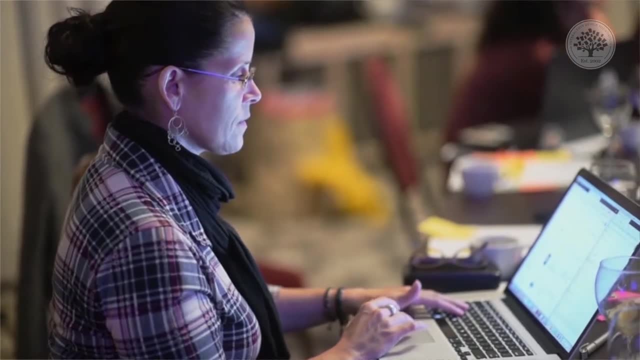 answer that you actually need to go out and research, understand, interact with real users. You need to do observation, so that's the watching them work, and I think observation is a fantastic tool and we don't really do enough of it. Research we can do in many, many ways, including. 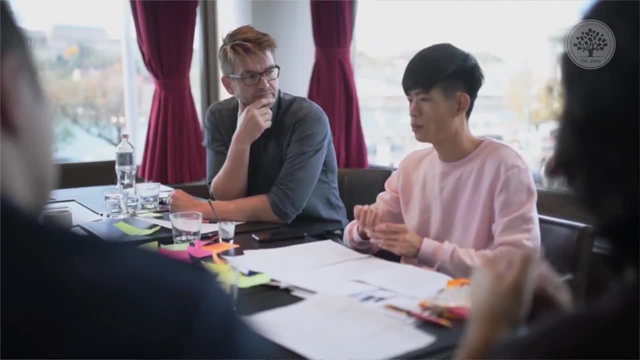 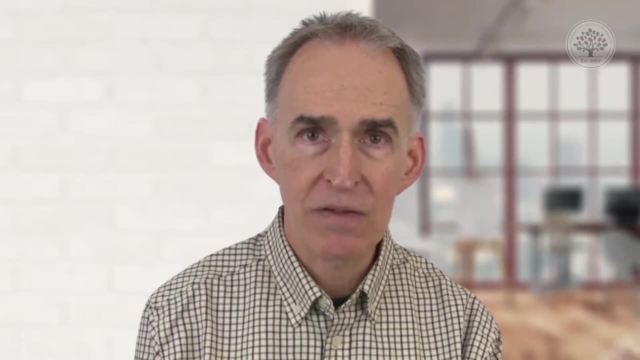 questionnaires and interviews, perhaps not quite as effective as observation, but they have their advantages in many cases. And then, finally, evaluation, and that's really key. If you did none of these other things, then evaluating with users would at least give you an idea whether you've got. 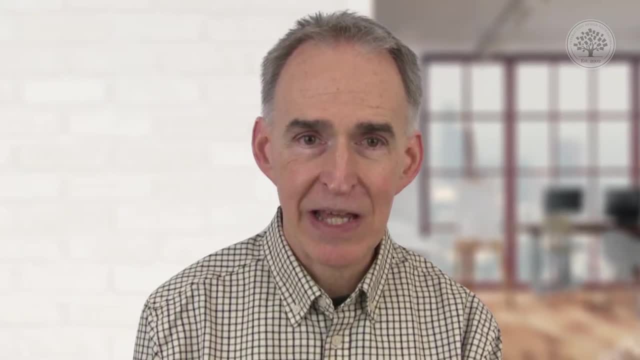 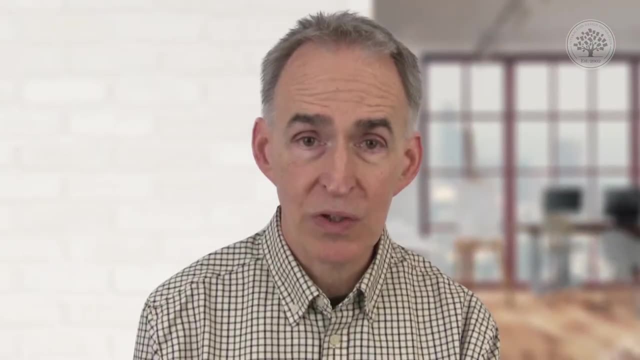 problems or not, But the argument I'm going to be making is that evaluation on its own is really a fairly poor solution to the overall problem that poor usability comes from. So let's have a look at some of these other points We need to research and 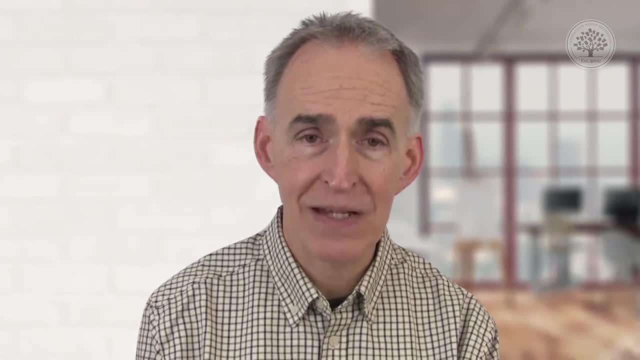 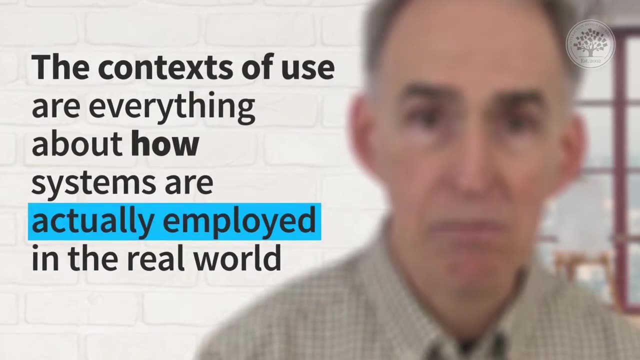 understand the context of use. It's a very powerful label because it really is fairly self-descriptive. The contexts of use are everything about how systems are actually employed in the real world, and I'll give you a couple of examples. One is the differences. 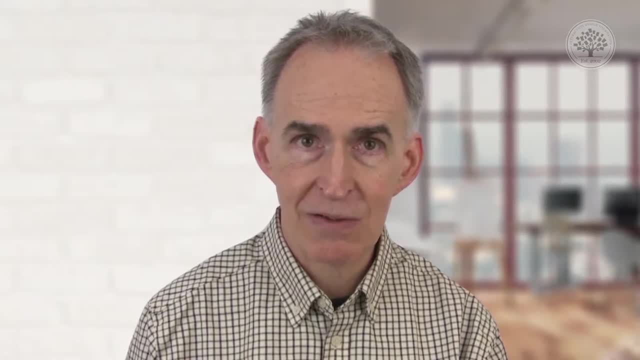 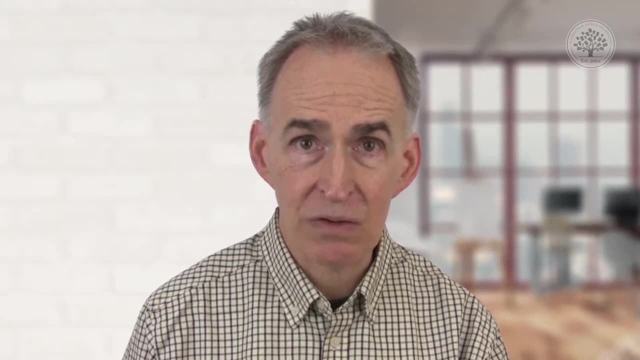 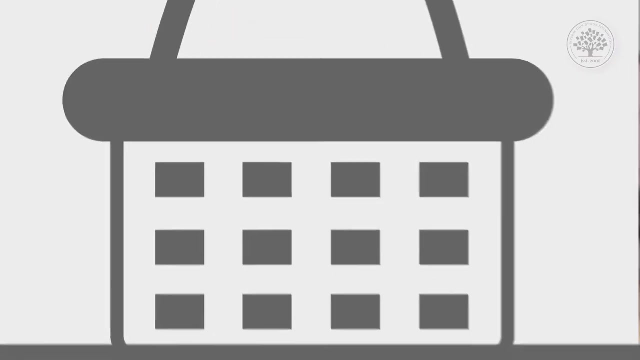 in use in the context of use between a point-of-sale system in something like a pub or a cafe versus a supermarket. The equipment may be virtually identical, The software might be very similar too, but the actual use of these systems could not be more different. In a supermarket, you have one. 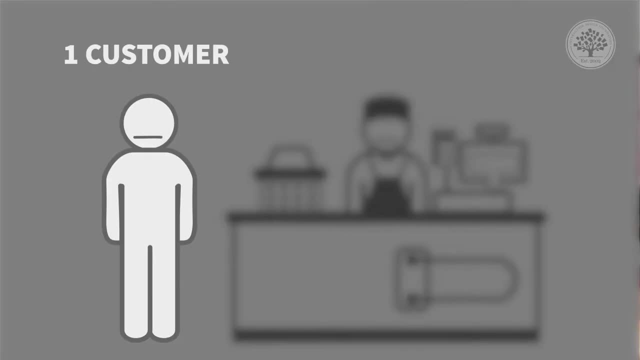 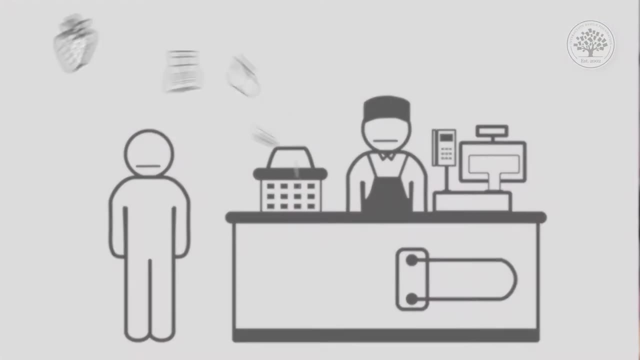 customer at a time, the person that you're actually doing the checking out for- and there is one user at a time. The user is the checkout operator and that person might have to go through a hundred or more times a day, and that person might have to go through a hundred or more times a day and that 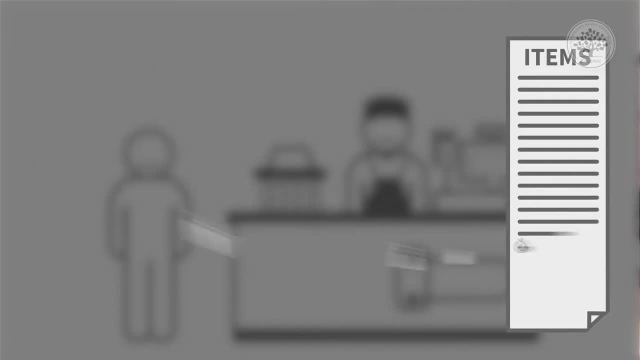 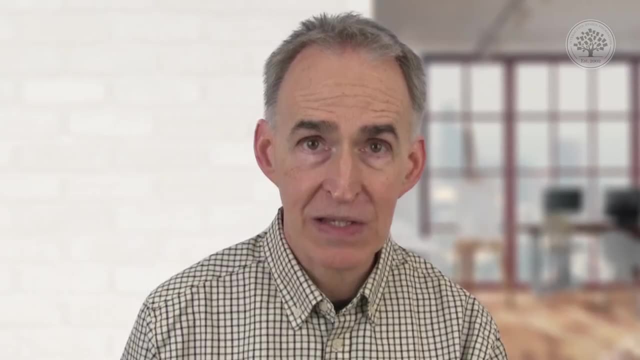 person might have to go through a hundred or more times a day and that person might have to go through a hundred or more items from somebody's weekly shopping. but important factors there are that it is just one customer and it is a lot of items and it needs to be done pretty efficiently And there aren't any. 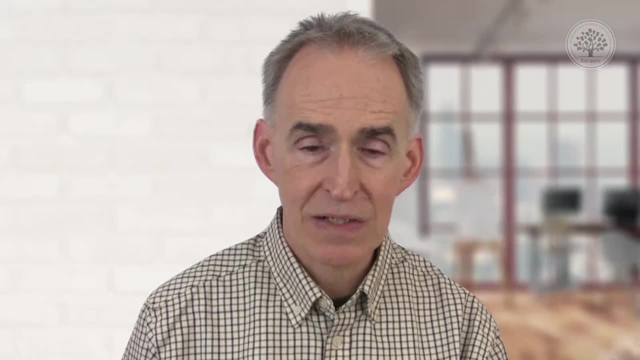 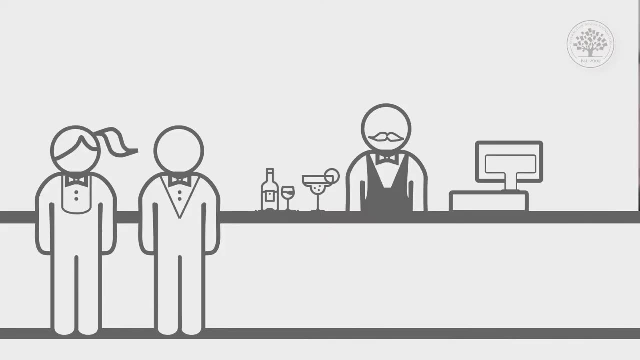 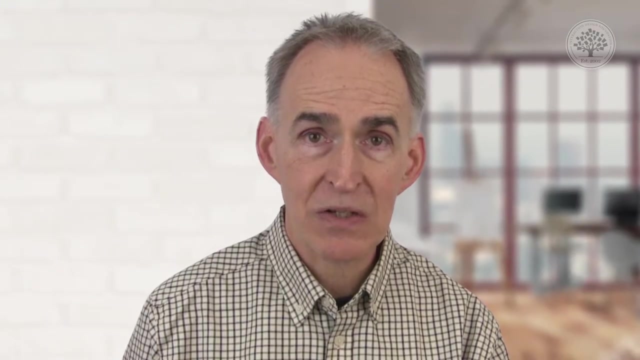 complications, typically from needing to change to a different customer midway through the process. On the other hand, the situation is entirely reversed. in a pub or a cafe or something similar, You have many people sharing the one point-of-sale of sales system And they need to be able to switch between customers very quickly. They need 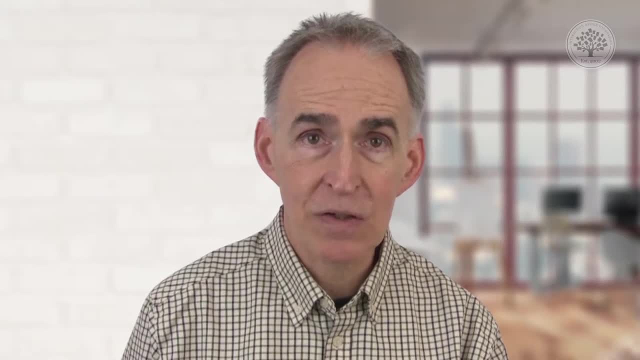 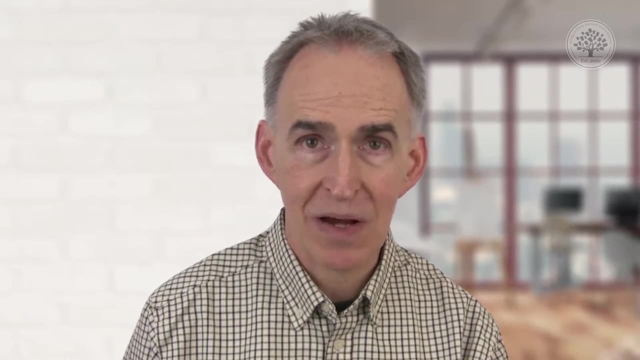 to switch between users very quickly too, And the whole thing couldn't be more different. And if you were to try to impose the supermarket system in a cafe or the cafe system in a supermarket, you probably just wouldn't get away with it. It just would be a horrible, horrible failure. 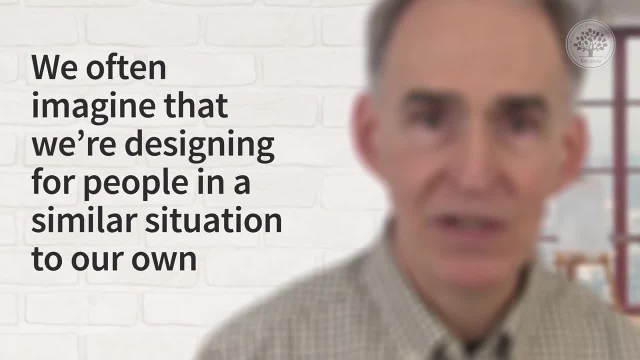 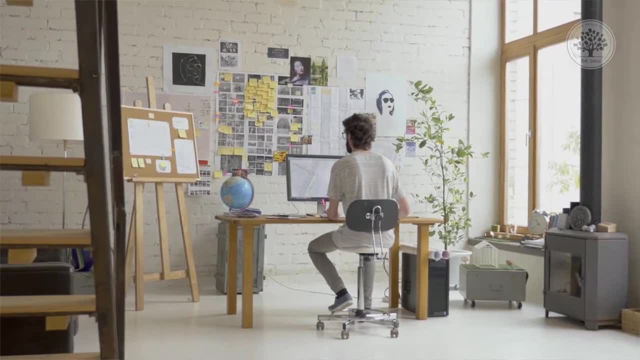 Other issues to do with context of use. We often imagine that we're designing for people in a similar situation to our own, where, for example, we're in a clean, dry, warm environment, typically an office environment. But as soon as you start looking further afield, as soon as you start, 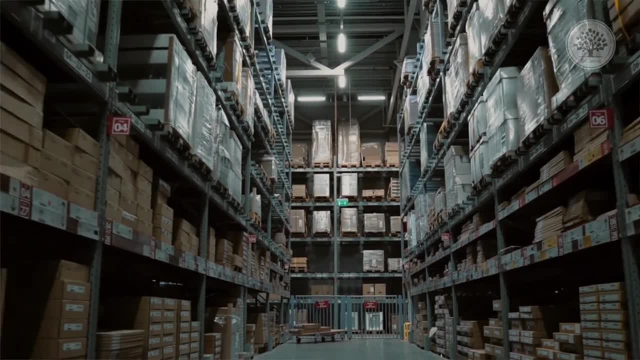 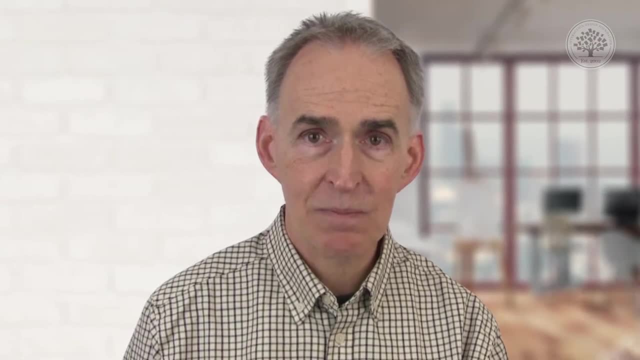 looking at warehouses or factories, then the context of use are very different And you need to design your systems differently. Sometimes it means using different hardware, Sometimes it means just being aware of the context of use in terms of how you write the user interface or how you 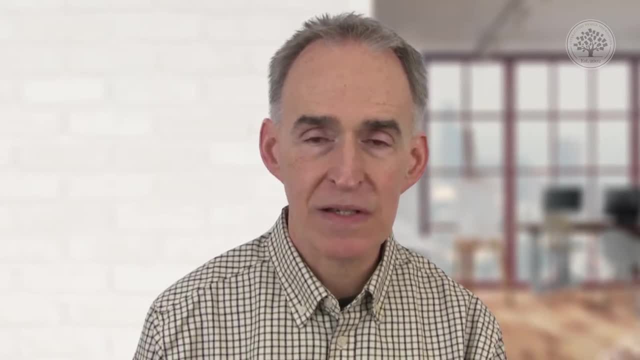 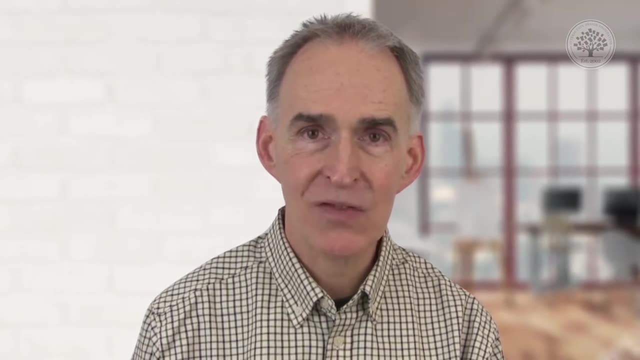 design the user interface. So the main focus of the context of use is how you write the user interface. The main focus for user-centered design is the suitability of solutions for real users in real contexts of use, not the ones that we are imagining. 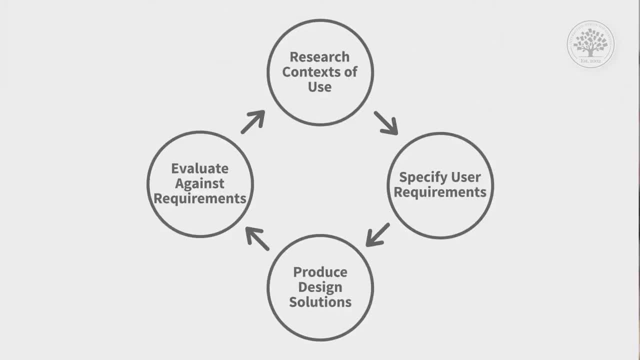 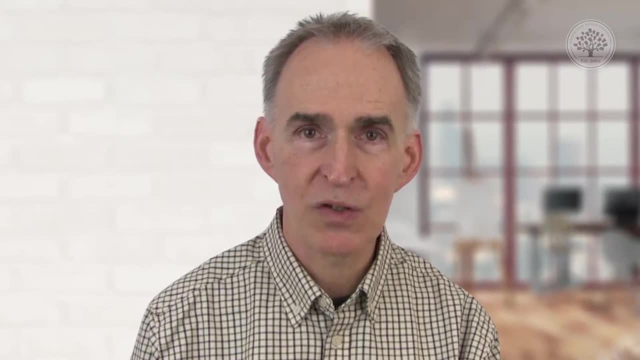 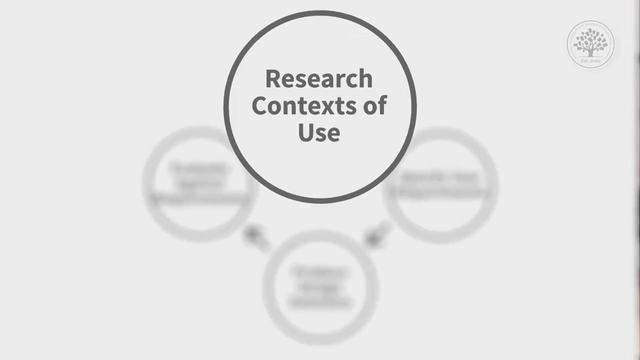 It's a fairly straightforward diagram really. We start with identifying the need for user-centered design, And I've actually left that off the chart because in my view, if you're creating interactive systems, you need to use user-centered design. So we start at the top with research context of use. We go around to specifying the user. 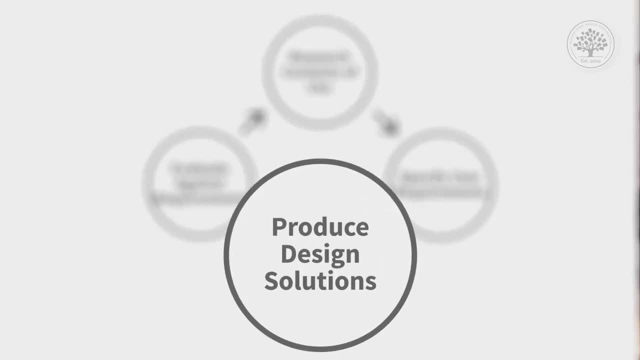 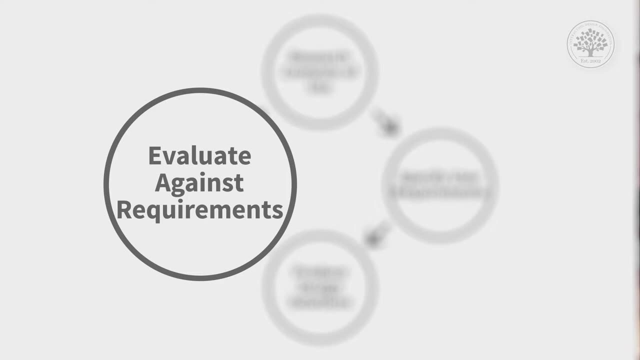 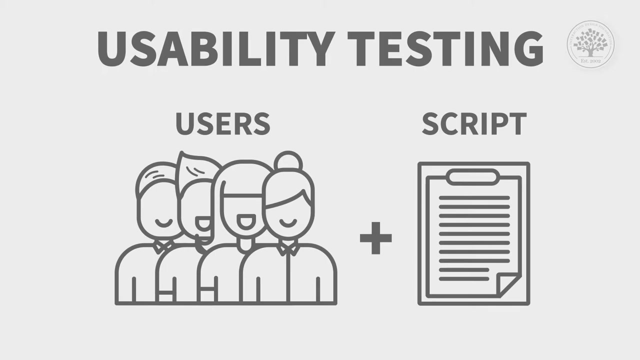 requirements. We finally, at the bottom, produce some design solutions And then, at 9 o'clock on the clock here, we evaluate those solutions against the initial requirements. And we do that with a number of tools, But one of those, of course, would be usability testing, testing with 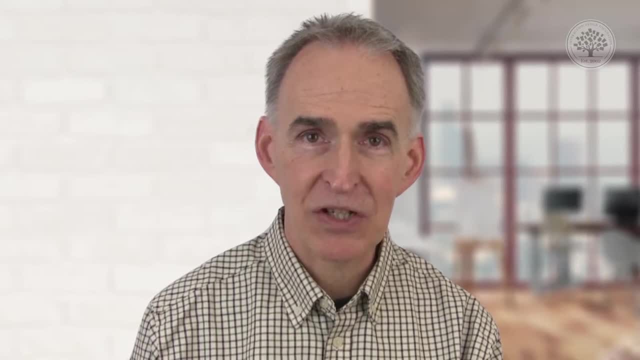 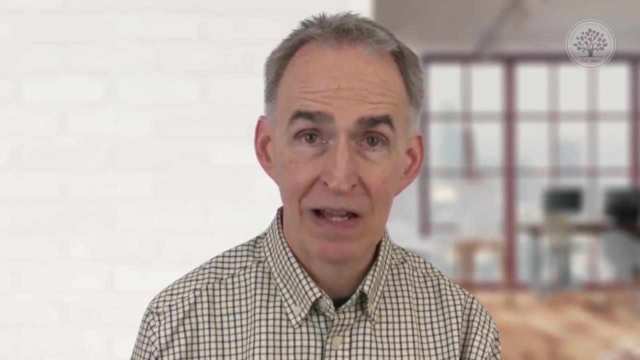 real users And, depending on how that goes, you might have to go back and start again with your context of use. This has certainly happened to me in more than one occasion that a customer that I've been developing software for has not told me about a context of use And we've only found out about it during testing. 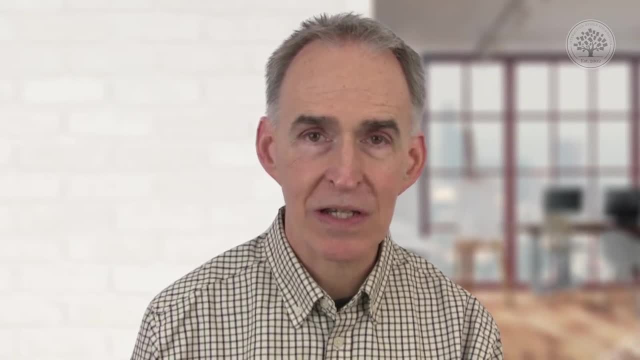 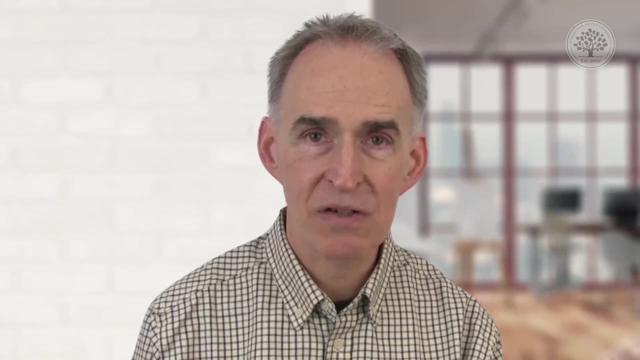 which is a little bit late in the day, Or you might have to return to just adjusting the user requirements. Hopefully you only need to go back as far as tweaking the design solution, So you go around that loop until you can come out on the left-hand side here with the meets requirements box. 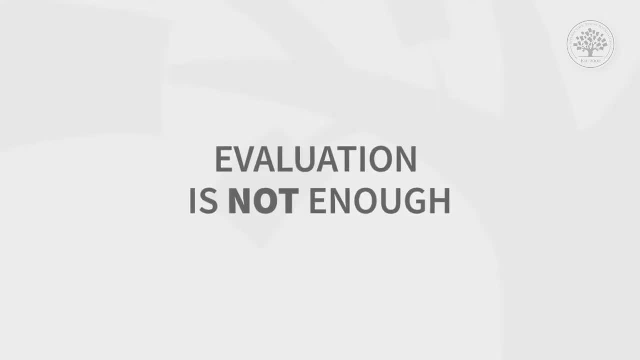 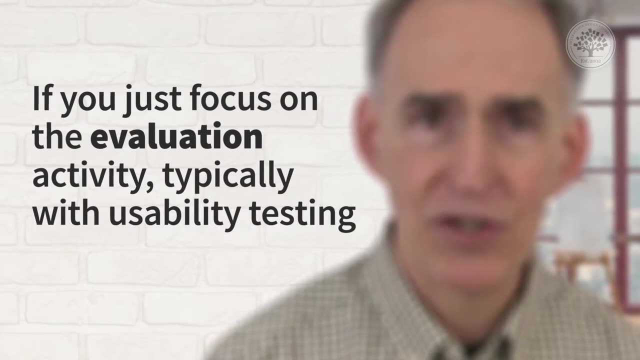 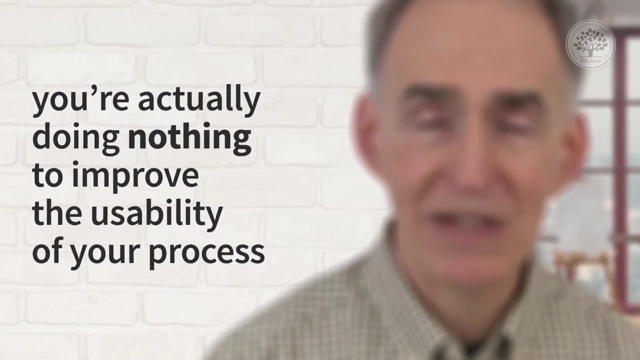 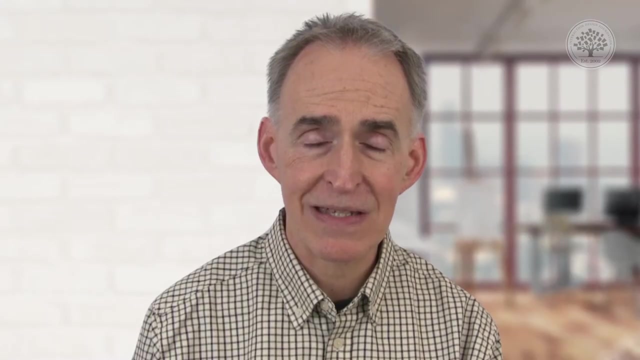 on that particular design. The main point I'm making about this is that if you just focus on the evaluation activity that I've marked here, typically with usability testing, you're actually doing nothing to improve the usability of your process. You are still creating bad designs, And just filtering them out is going to be fantastically. 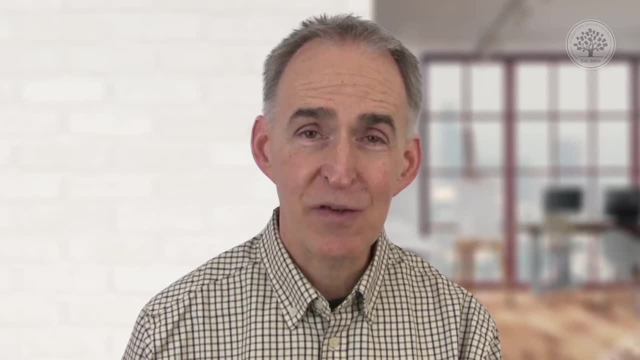 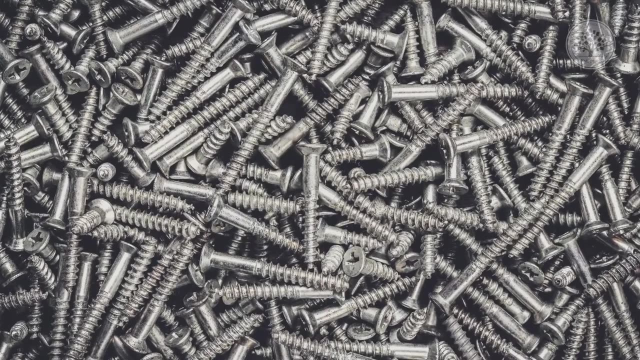 wasteful in terms of the amount of effort. So if you think about it as a production line, we have that manufacturing analogy and talk about screws. If you decide that your products aren't really good enough, for whatever reason, they're not consistent. 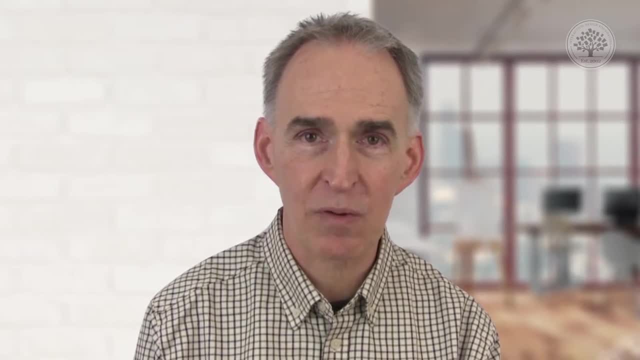 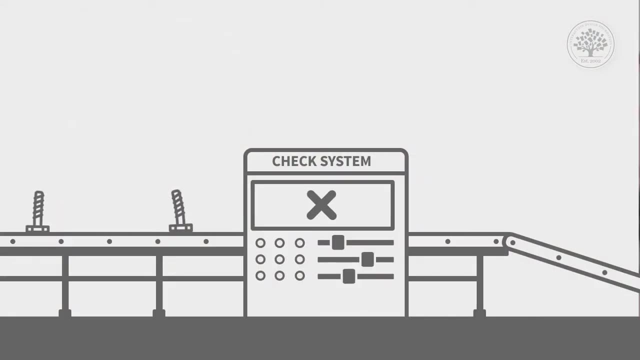 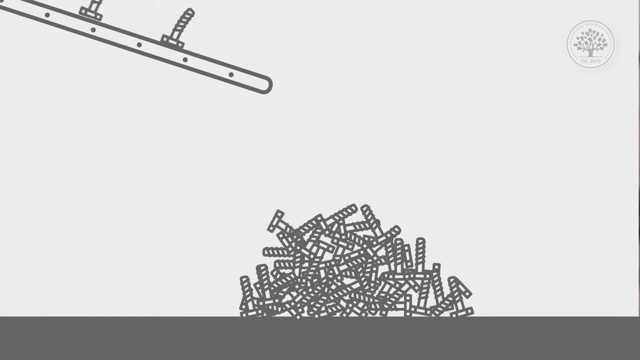 or they break easily or any number of potential problems, and all you do to improve the quality of your product is to up the quality checking at the end of the assembly line. then guess what? You just end up with a lot of waste because you're still producing a large number of faulty screws. And if you do nothing to 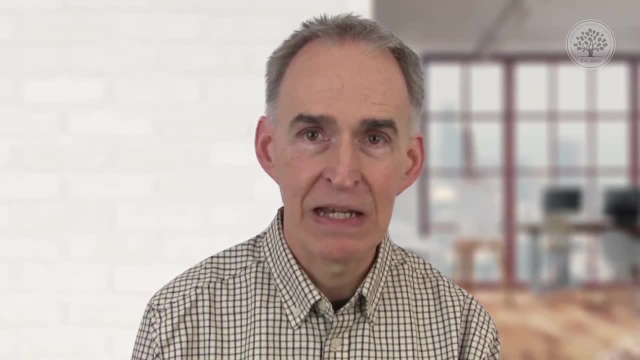 improve the actual process in the manufacturing line. you're still producing a large number of faulty screws. And because you're still producing a large number of faulty screws, then guess what? You're still producing a large number of faulty screws. And because you're still producing a large number of faulty screws, And because you're still producing a large number of. 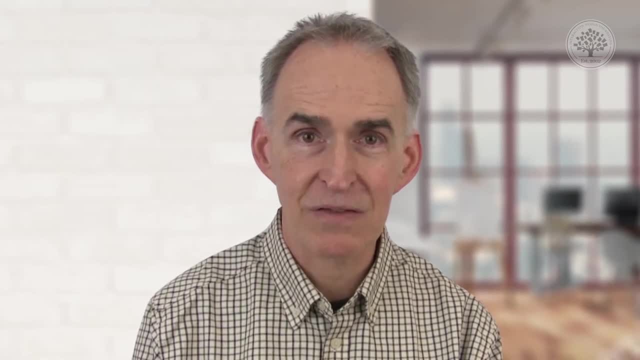 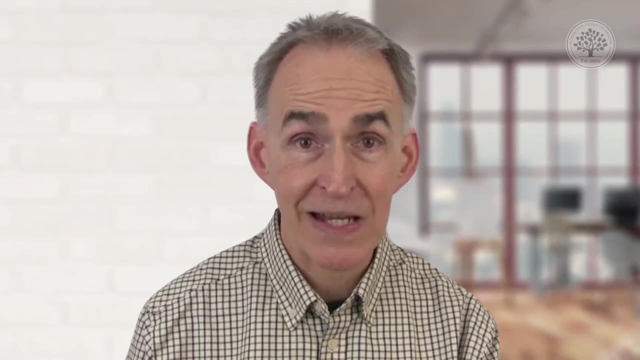 faulty screws And because you're still producing a large number of faulty screws, then just tightening the evaluation process, raising the hurdle effectively, is really not the way to go. Use Ability evaluations are a very important tool — usability testing in particular is a very important tool in our toolbox, But really it cannot be the only one, And that's. 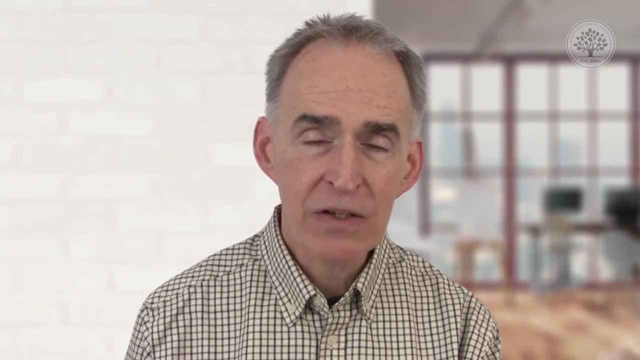 something that we need to take into consideration at the outset. The other issue I should mention is that often we miss things. We didn't realize when we designed this that there would be variables in the software that would force us to apply a step in the wrong direction, and that's not always the case, And if you have a good enough tool, you don't lose that ability. 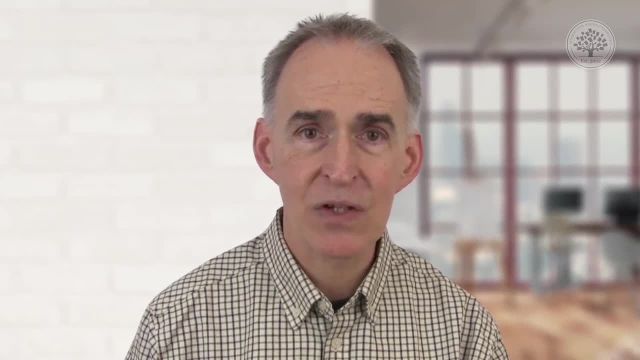 users or customers in particular contexts of use that needed slightly different requirements. I remember a project where I was discouraged from talking to a particular user because the business saw him as troublesome. He's actually an internal user, it wasn't an external customer, and the reason it 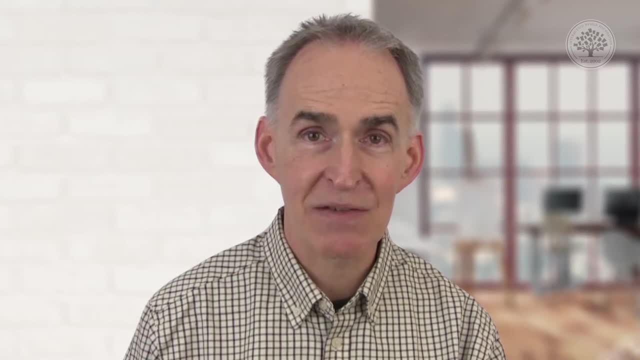 turned out that he was troublesome is that his needs were different to most of the other needs of his colleagues in the organization, but it was for a good reason. He was responsible for a particular market and that market was just different to the rest of the markets for that organization. So we 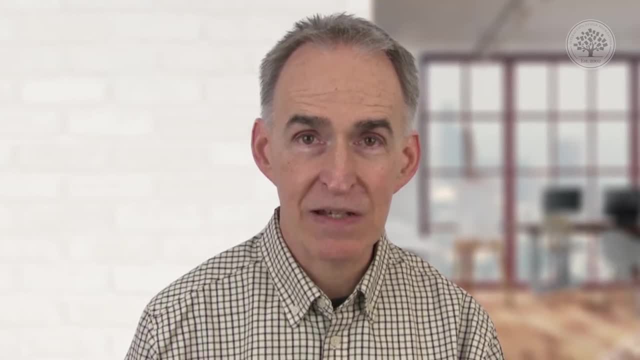 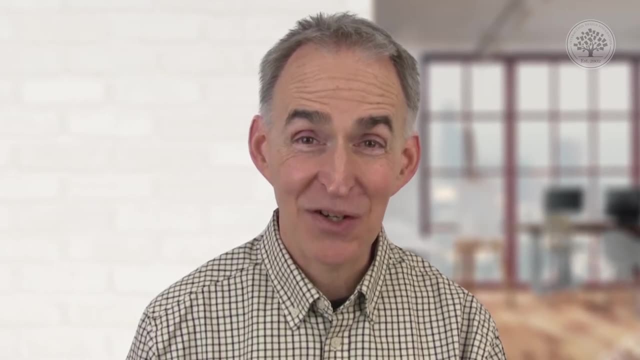 didn't think to build a solution that catered for his needs and of course, when he came to start using it he said: but how do I, or where is, and all kinds of good questions like that, and it was just absent And of course you can't do. 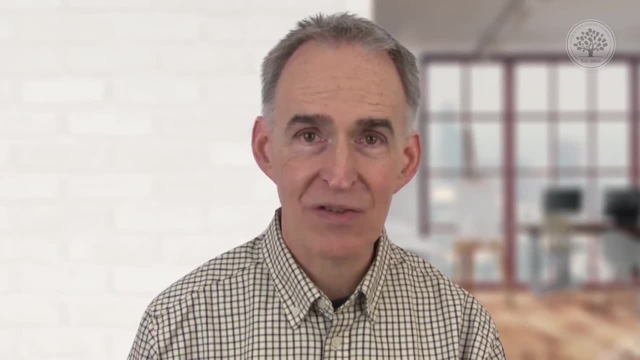 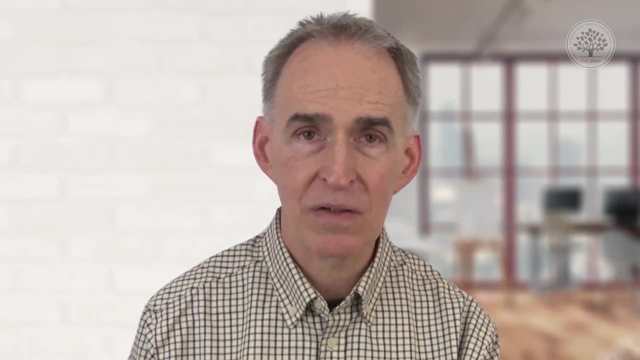 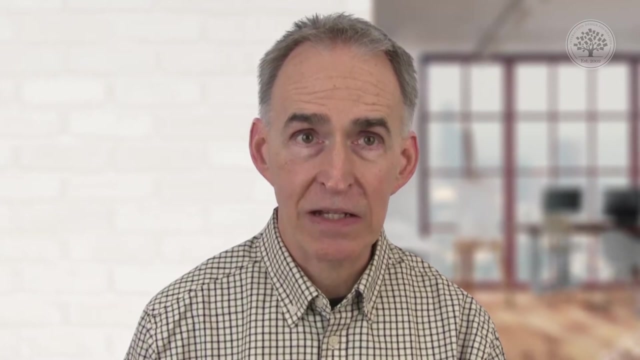 usability, testing on things that you, or evaluation on things that you've actually not built. So there is another good reason for making sure that your process is focused. It's focused on users rather than just your evaluation. A summary of steps to take in user-centered design, and this is what's talked about in the International 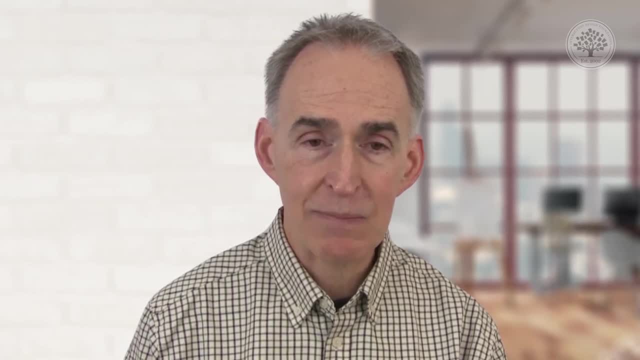 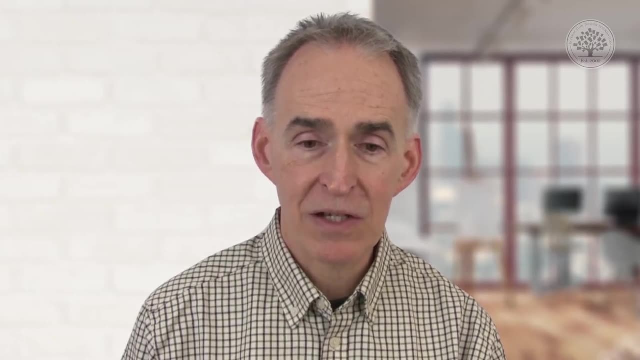 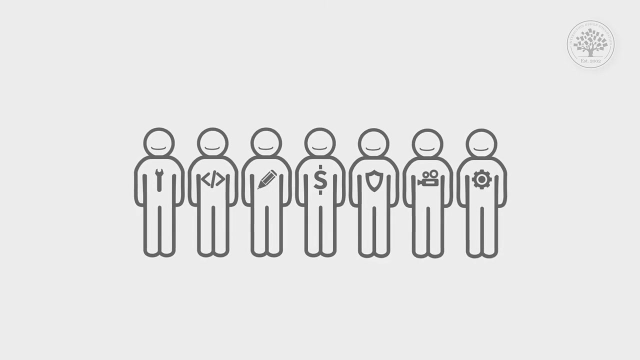 Standard multidisciplinary teams. You will get people who are not focused strictly on technology, so you might well improve empathy. that way You might certainly get better problem-solving, because having people with different kinds of backgrounds or expertise is a much better way of solving problems than 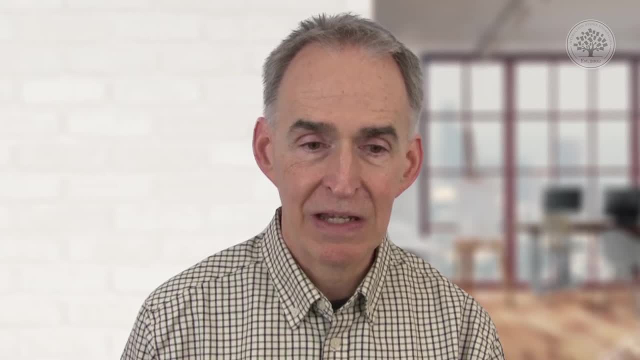 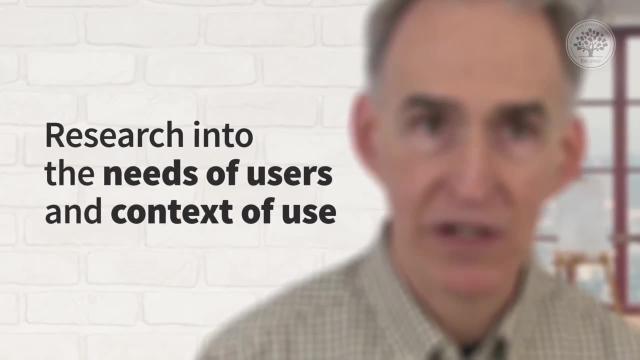 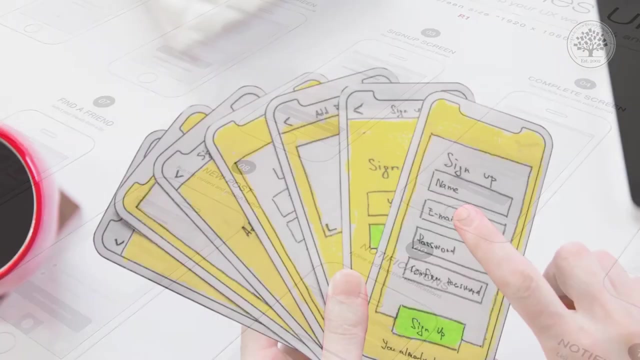 a lot of people who don't know how to solve problems. We need to research into the needs of users and their context of use. We need to produce prototypes as early as possible, but we need to produce prototypes, perhaps low fidelity prototypes, paper prototypes even- and just make sure that our ideas. 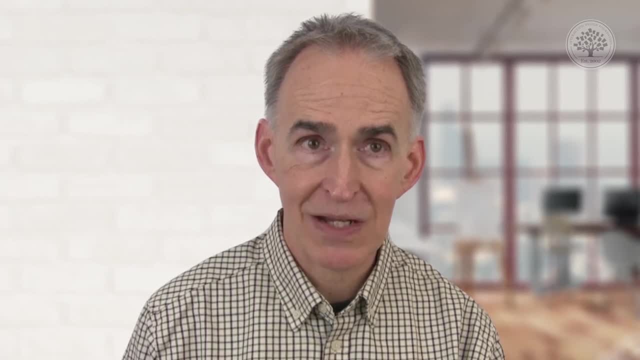 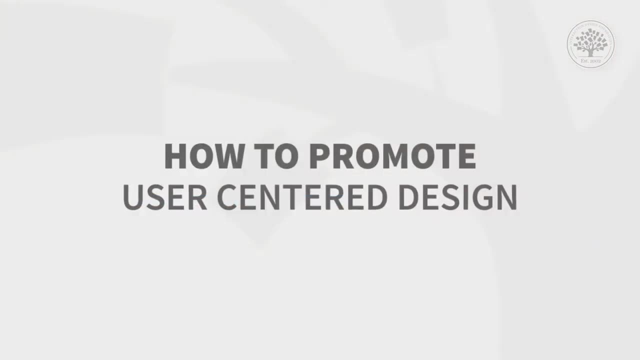 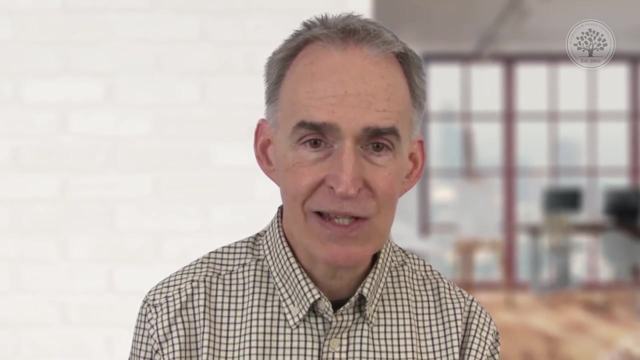 are sound and we need to test those realistically with potential users. Last but certainly not least, we need time scales to allow feedback and design changes. what do we need to do? well, make all team members aware of the basics of designing for users, and I think that's key. I think it's not very helpful to 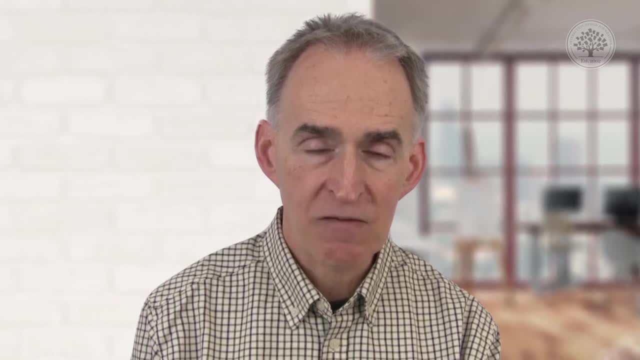 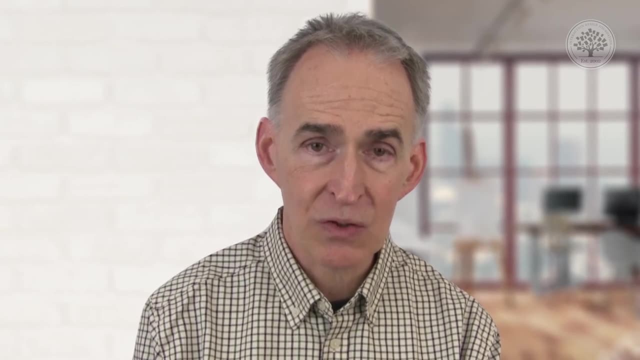 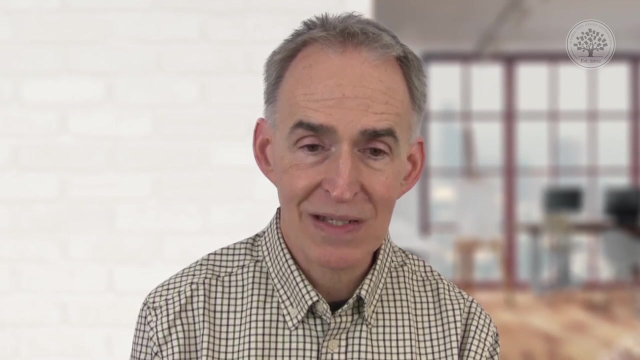 have people who don't understand why. we need to have personas to understand why we need to consider solving this problem for other people- these people who are perhaps not so good at systemizing or understanding systems. we need to improve awareness of user focus, design tools and techniques so that people can.